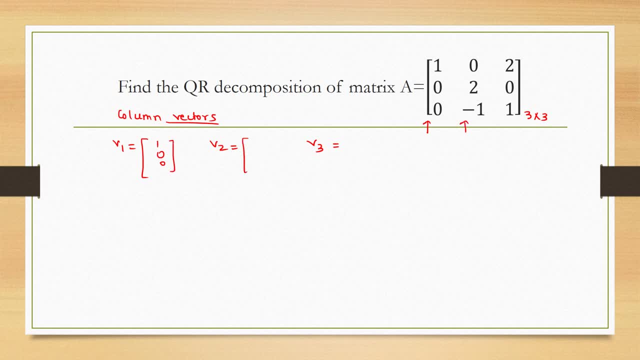 Third column is 2,, 0,, 1,. right Now you have to find out orthonormal basis. Orthonormal basis, just like you did it in Gram-Smith process. So how you do that? Firstly, to get orthonormal basis, you have to find out orthogonal basis using Gram-Smith. 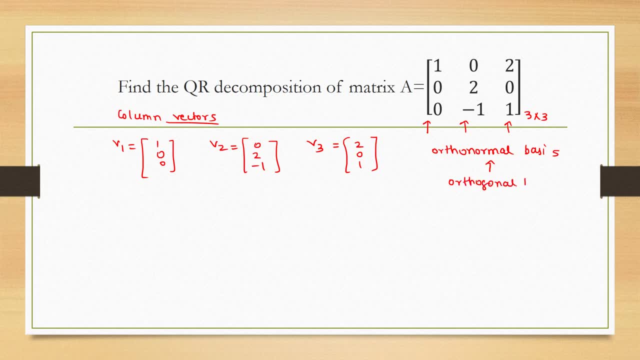 So I'm telling you how you can do that. You can do so, So you? because there are three column vectors. so there will be three orthogonal basis. Let's say Y1, Y2 and Y3. Y1 is always equal to the first column vector, which is V1. here, that is 1, 0, 0.. Now what about other two, Y2 and Y3? The formula which Gram-Smith says is: Y2 is equal to V2 minus dot product of V2, Y1.. 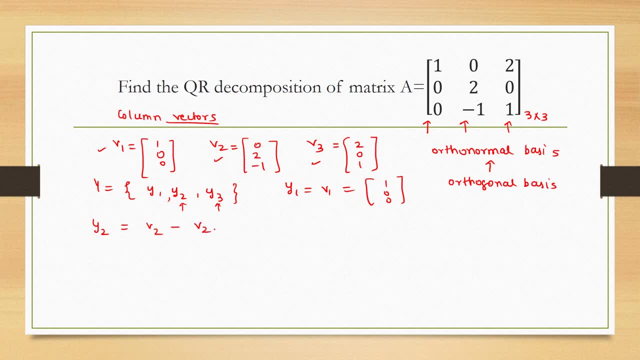 Then V2 is equal to dot product of Y1, Y1 and its whole dot product with Y1.. So if we calculate it separately, V2 dot Y1 is what. V2 is 0 to minus 1 and Y1 is this 1, 0, 0.. So do the dot product. 0 into 1 is 0.. 2 into 0 is 0.. Minus 1 into 0 is 0. So this is 0. So we don't need to calculate anything. 0 multiply with anything is 0. So only V2 is left. 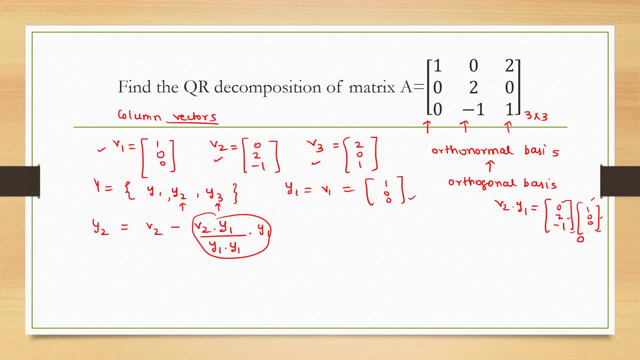 Now for Y3, what we have is the formula is Y3 minus, I mean V3 minus V3- dot V1, V1- dot. V1 and its dot product with V1 minus V3. dot. V2 divide by V2- dot. V2, its dot product with V2.. 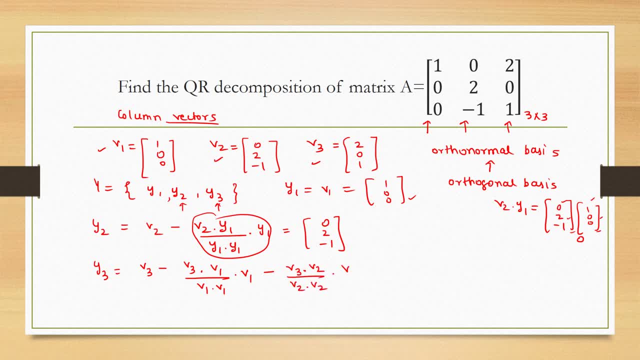 So here we have V3 as 2, 0, 1 minus V2.. v3.v1. we can calculate here: 2 0 1 and v1 is what 1 0 0. so 2 times 1 is 2, rest all will be 0. 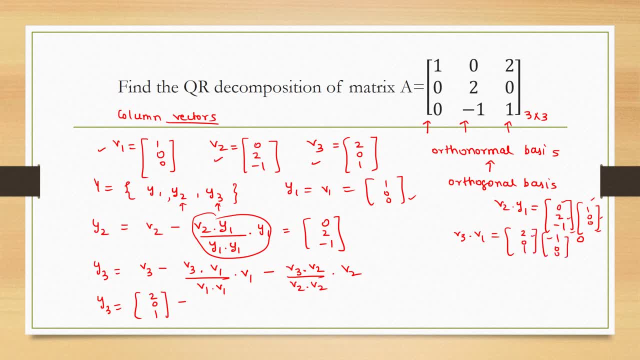 so this is 2, correct then. v1.v1 is what v1.v1 is 1 0 0 dot 1 0 0. so 1 times 1 is 1, right. so this is 2, this is 1, so 2 by 1 is 2. v1 is 1 0 0 minus. v3.v2 is what v3.v2. 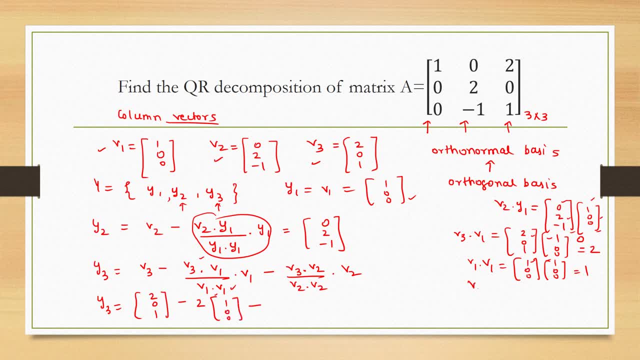 v3 is 2 0, 1 and v2 is 0, 2 minus 1. so this 2 times 2, 0 is 0, 0 times 2 is 0, 1. dot minus 1 is minus 1, and then we have to find out v2.v2. so 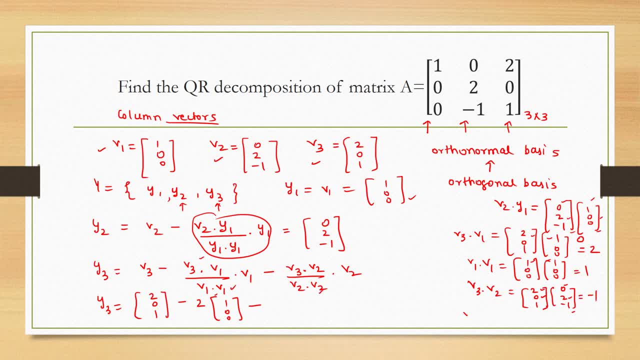 so. so v2 is 0, 2 minus 1, 0, 2 minus 1 0 times 0 is 0, 2, 2 is a 4 minus minus plus 1, that is 5. so v3.v2 is here minus 1. 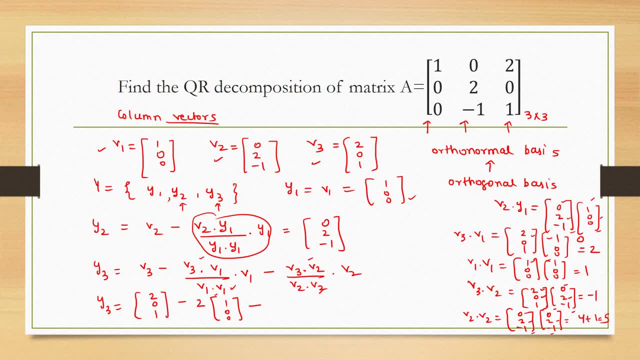 divide by v2.v2 is 5, and then we have v2, which is 0, 2 minus 1, right? so this form, this form Butterfly, forms two zero one minus two, as a two zero zero Minus two, zero, one minus k plus one by five. 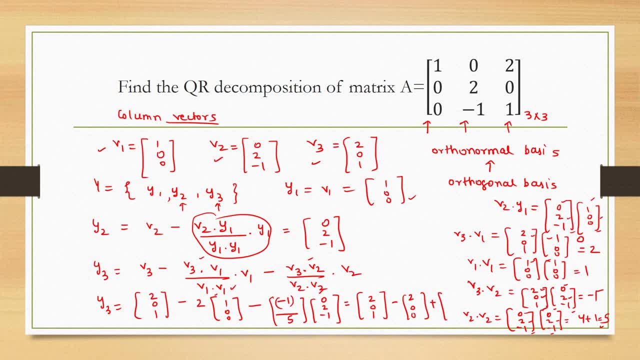 So if you multiply one by five with zero, 0, 0, this is two by five, then minus one by five. Correct, now you have to calculate the rest. so first element will be 0. let me change the pen so that you can clearly see it. 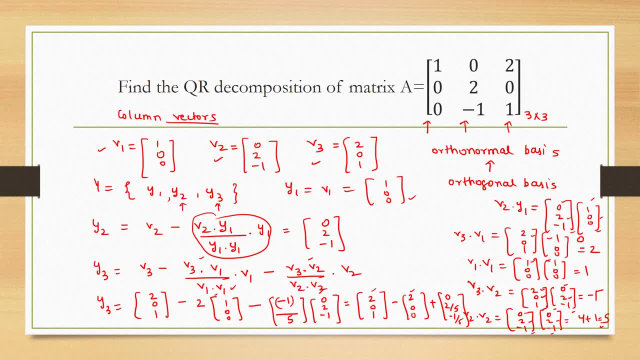 2 minus 2 is 0. so first element is 0. 0 minus 0 is 0. only 2 by 5 is left, and 1 minus 0 is 1. 1 minus 1 by 5 is 4 by 5. so this is your y3. now you have your. 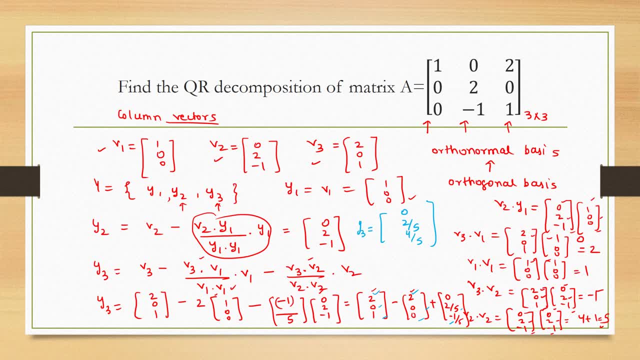 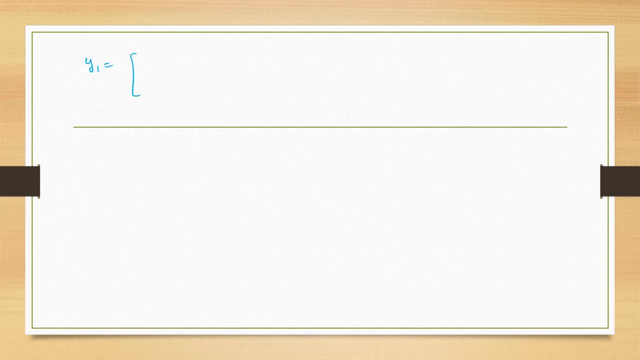 orthogonal basis how you will calculate your orthonormal vector. so let me rewrite y1, y2, y3. y1 is your v1. only that is 1, 0, 0, y2. we calculated 0, 2 minus 1 and y3 we. 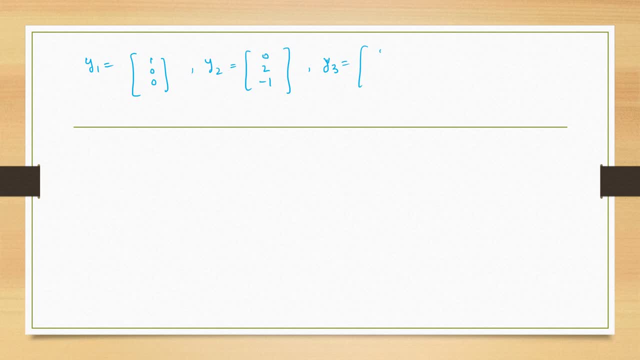 calculated as 0, 2 by 5. 4 by 5 right. y2. we calculated 0, 2 minus 1. and. y3. we calculated as 0, 2 by 5. 4 by 5 right. y3. we calculated as 0, 2 by 5. 4 by 5 right. 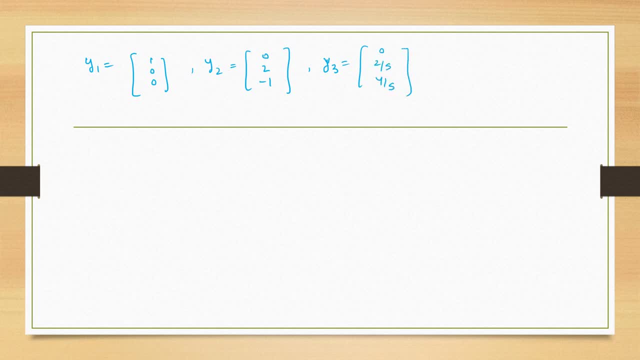 so these are orthogonal basis, right, in the form of y. now, in order to get orthonormal basis, what you are supposed to do, you have to divide orthogonal basis with the norms. so norm of y1 will be- it's like modulus 1 root, 1 square plus 0 square plus 0 square, so only 1 will be there then for 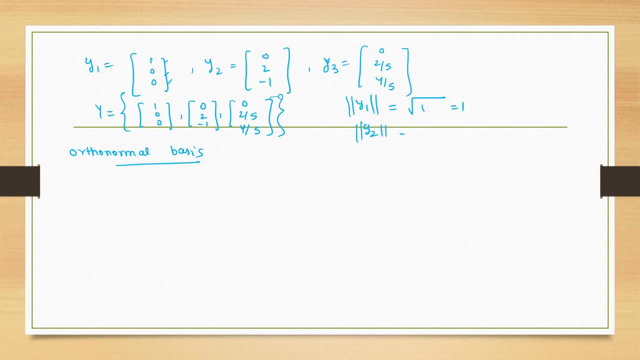 y2 you have 0, square is 0, 2 square is 4 minus 1, square is 1, so root 5 and for y3 it is 0, square 2 by 5 whole square plus 4 by 5 whole square, that is 2 to the 4 by. 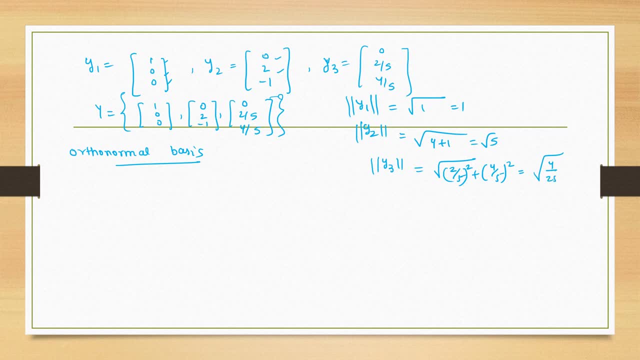 25 for 4, the 16 by 25, 20 by 25, 5. 4s are 5, 5s are 2, by root 5, so just divide. orthonormal basis will be a set of these orthogonal basis divided by the norms. 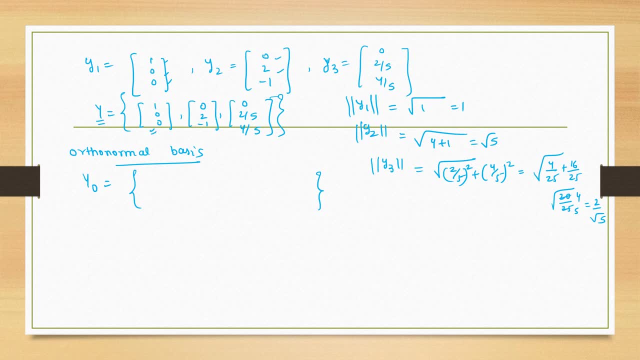 their respective norms. so y1 divided by modulus of y1, it is 1 only, so it will be same. so y2 divided by norm of y2, that is 1 by root 5 divided with, divide root 5 with all the elements, 2 minus 1. I mean divide all elements with root 5 and then 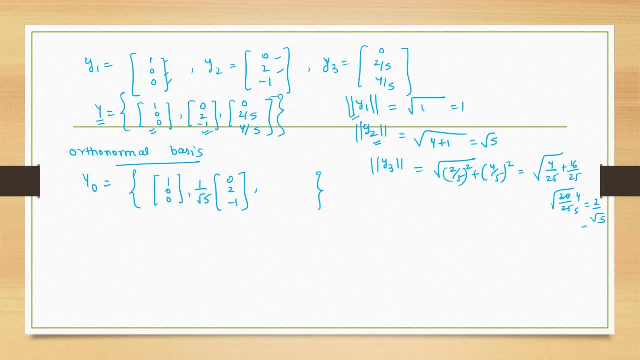 for third one, we have 2 by root 5, right? so 1 by 2 root 5. 2 by root 5. so root 5 will become numerator 0. 2 by root 5. this is only 5, right, let me use it is 0. I'm hoping you are getting it right. 4 by 5, but this is like. 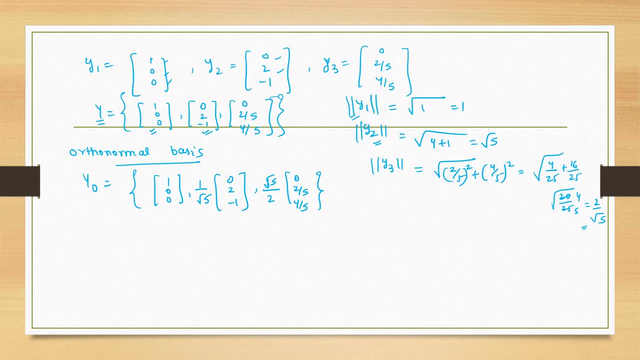 you have done this question up till Gram-Smith process, but now you have to decompose that matrix into QR, right? so what is Q? Q is basically the matrix form of these orthonormal basis. that is 1: 0, 0. if you divide 1 by root 5 with these. 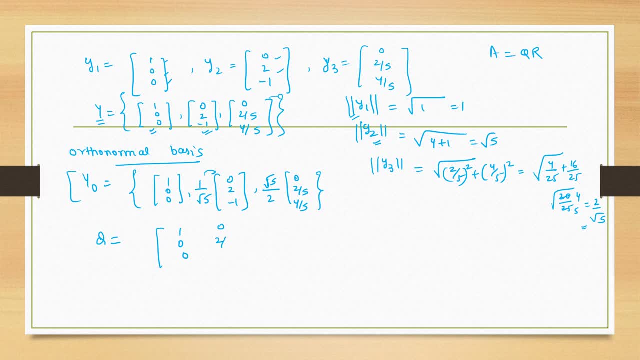 orthonormal basis, that is 1 0 0. if you divide 1 by root 5 with these orthonormal basis, that is 1 0 0. if you divide 1 by root 5 with these 0, 2 by root 5 minus 1 by root 5, and then this is 0. if you divide 2 by 5 with: 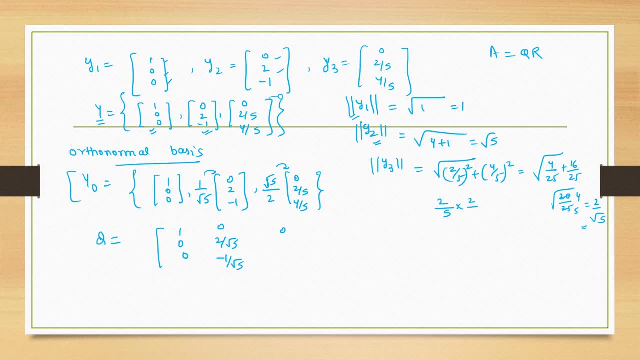 the root 5 by 2, it will be 4 by 5 root 5, right? just bear with me. it is 2 by root 5, right? so it was 1 by 1 by 2 by root 5. so it becomes like this: okay? so if you? 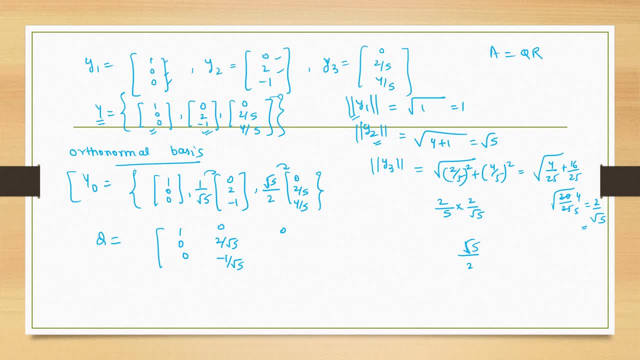 just simply multiply this. you have already divided, right, so just multiply 0, then 2 by 5 into root 5 by 2. this is nothing. so you can split root 5 as root 5 as root 5 into root 5. right, so it is 2 by 2 root 5, right, then you have 0 here. okay, 2 can also be. 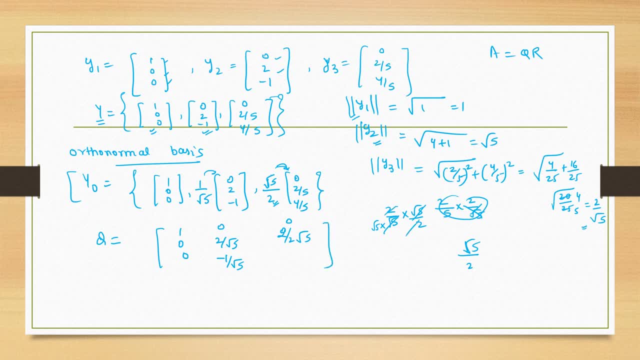 cancelled, just bear with me. so now all we get one by root 5 only right. then if you do root 5 by 2 x 4 by 5, difference of 4, and then 1 root 5, so 2 by root 5. this is your q. 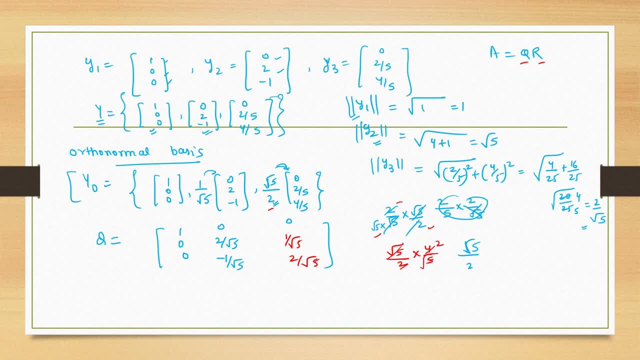 now you have to find out other metrics, which is are, because of course this is Qr decomposition, right? so what is our now? so you calculate by the keys on all your. so you calculate r using q transpose a. okay, so q transpose, that means make rows as column 1: 0, 0. 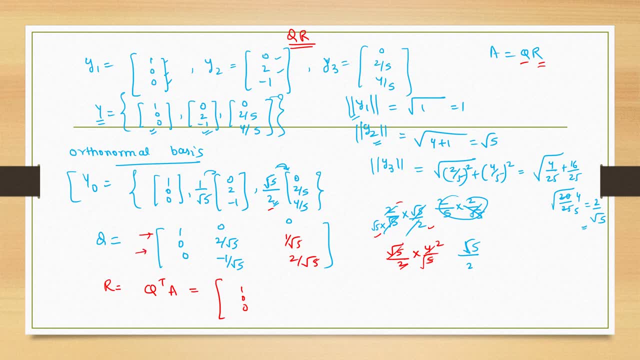 then second row will become second column: 2 by root 5- 1 by root 5. and third row will become third column minus 1 by root 5: 2 by root 5. this is your r and okay, this is q. transpose and a is: 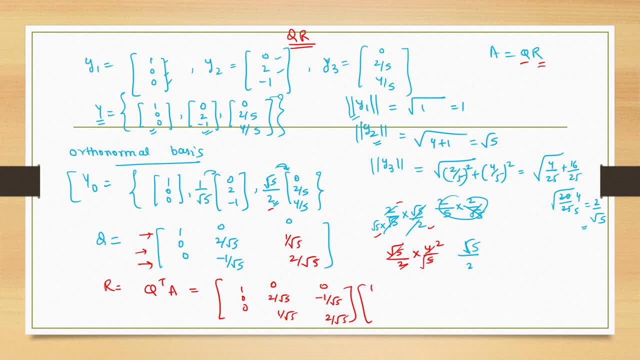 what a is your question matrix which is given in the question: 0, 2 minus 1, 2, 0, 1. okay, now multiply this. so either what you can do, this is your r matrix, right? first row, first column: multiply 1 times 1 is 1 and rest will be 0. then, first row, second column: 1 times 0 is 0, 0 times 2 is 0. 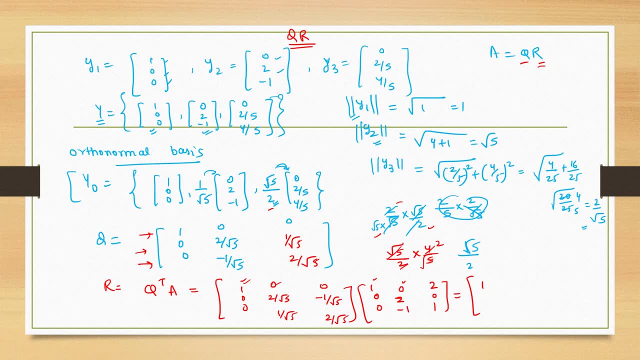 this is first row. second column is 0. then first row, third column: 2 times 1 is 2, rest all will be 0, right? so 1, 0, 2 is your first row, then second row. first column: this will be 0, only second row, second column, so it is a 4 by root: 5. 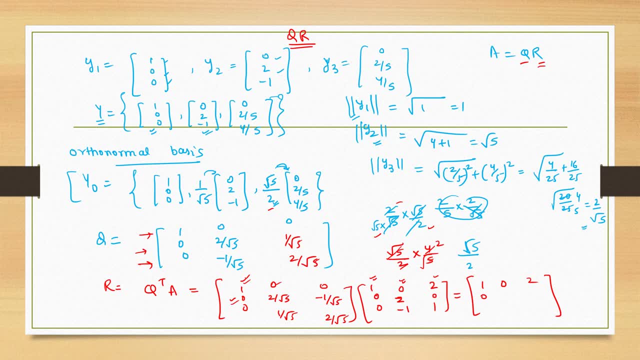 so 4 by root 5 minus 1 by root 5 into minus 1 plus 1 by root 5. that means 5 by root 5, that is root 5 only correct. then second row, third column: 0 times 2 is 0. this is 0, only minus 1 by root 5. then third row: 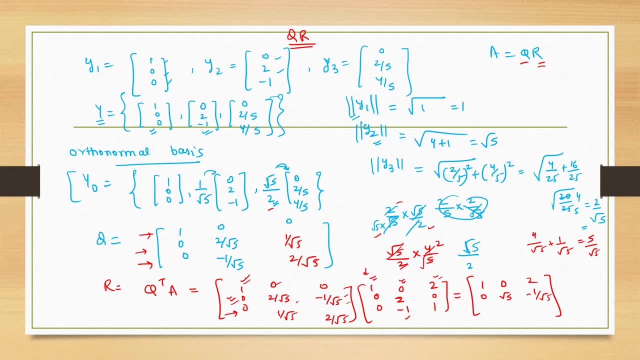 first column 0, this will be 0. then third row, second column 0: multiply 0 is 0, 1 by root 5 into 2 is 2 by root 5 and 2 by root 5 minus 1. so minus 2 by root 5, that is 0. 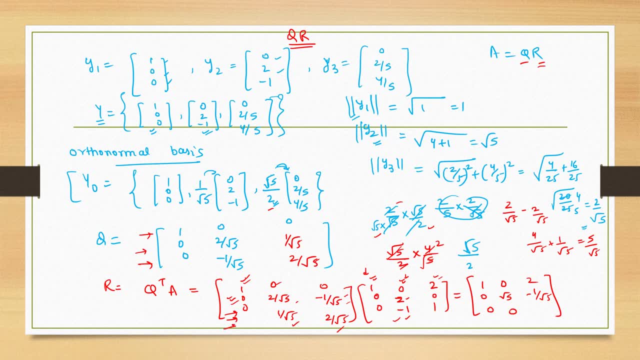